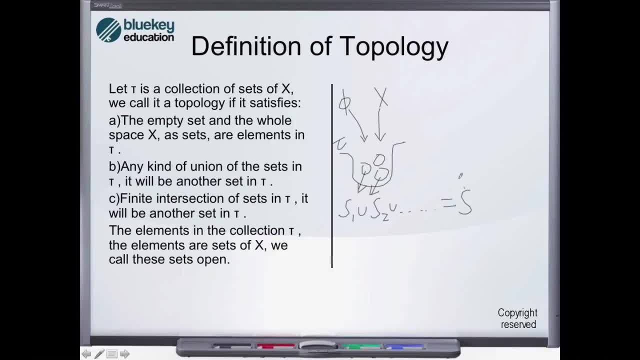 sets together, we will have come up with another set. We require that this set to also exist inside the bag. Similarly, if I were to take sets once again- so this time I'm only allowed to take finitely many sets, all the way to some number n, and then I choose to intersect these sets together- 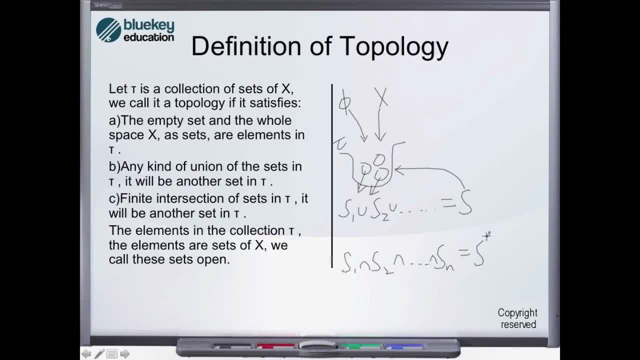 then I would have created another set, maybe call this set S star. then I would require that S star to also exist inside the bag. If this bag follows these three rules, then we call this bag a topology and we give a special name for the sets inside. we call these sets open sets. 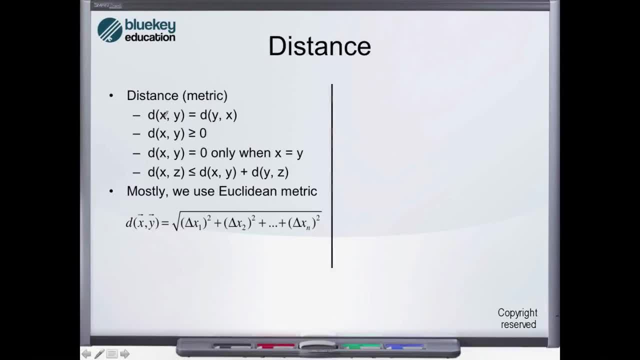 Sometimes we define a distance on a space. we require the distance between the first point and the second point to be equal to the distance between the second point and the first point. The distance must be always greater than zero. it's only equal to zero when the two points 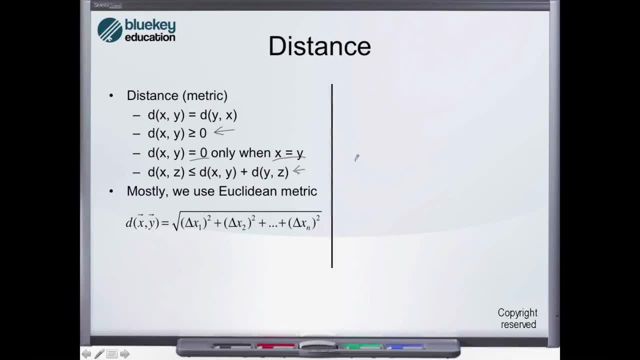 are equal and we also have the triangle inequality. pick any two points you like, call it x and z. and pick a third point somewhere else. call it y, Then the distance is equal to zero. The distance between x and z must be shorter than if I were to go to y first, then back. 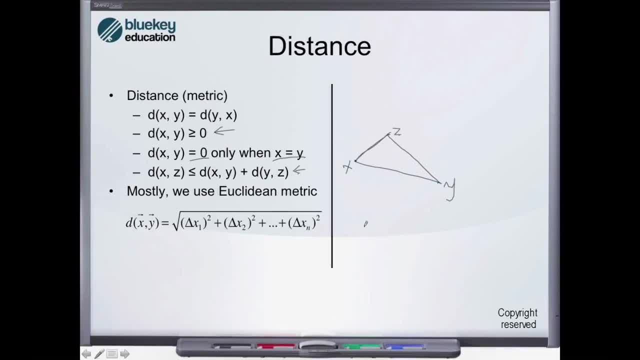 to the second point. We use the Euclidean distance mostly, which is a generalized version of the Pythagoras's theorem: the side length of the first one squared plus the side length of the second one squared, all the way to the last one squared, and then take the square root. 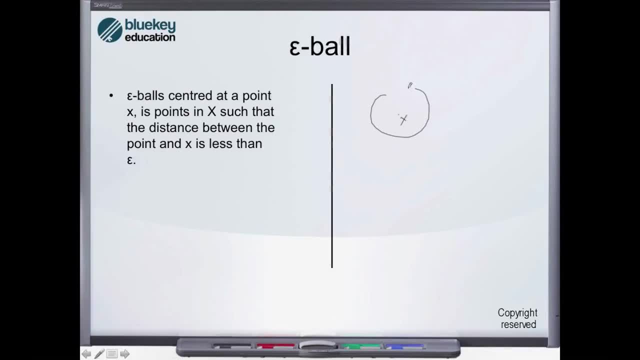 Pick any point we like in the space. we can define an epsilon ball around it, with radius being epsilon. The points inside the epsilon ball are precisely the points, such that the distance between the point and x is less than epsilon. So this point will be in the ball because the distance between this point and x is less. 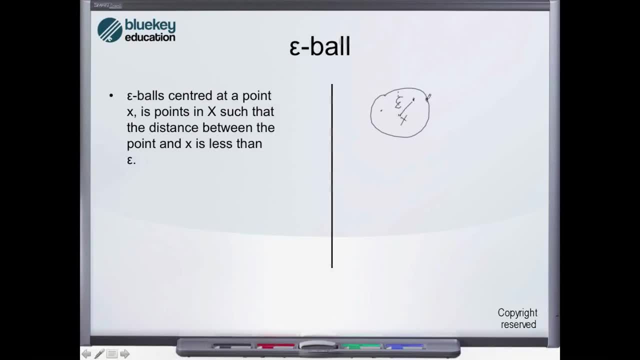 than epsilon. However, the point over here, exactly on the boundary of the ball, is not inside the epsilon ball, because the distance between this point and x is exactly equal to epsilon, which is not less than epsilon. Pick any set we like, call it c. 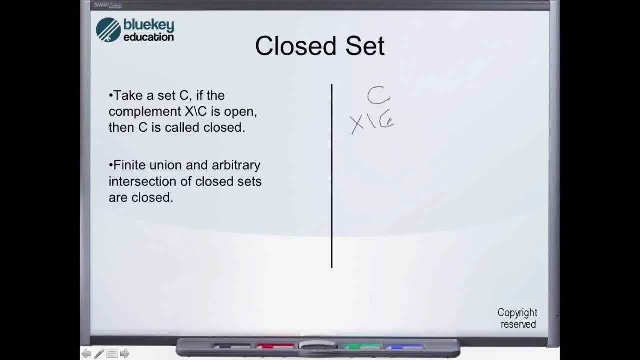 We don't have to do the same thing over and over again. We just have to define the distance between the point and x. We define the complement of c as saying every point inside the space that is not c. If this complement turns out to be open, then we call the set. we started with a closed set.